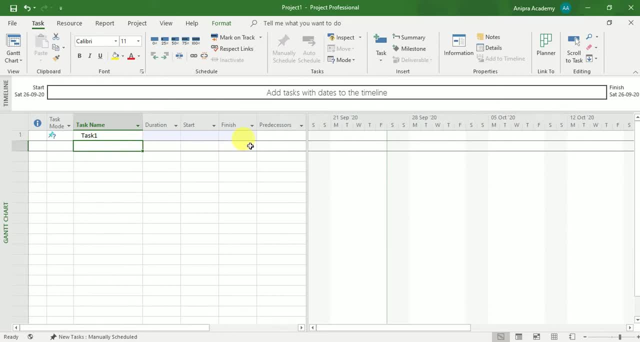 So here you can see the duration is start- finish. Everything is the amputee. and suppose, from here, if I will select the auto schedule right, Then if I will say this is my task number two, Then you can see duration is start and finish. 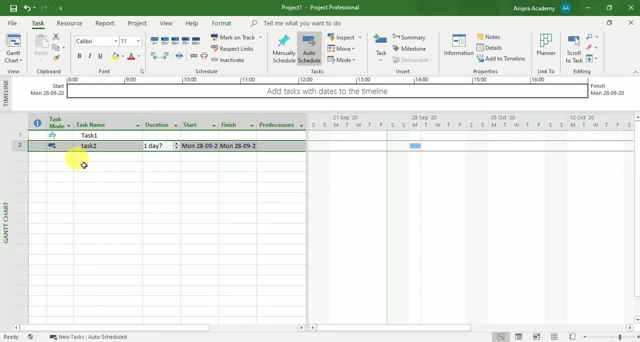 Finish date: auto populated, right. So if you want you can just do it from here also, okay. so this is the manual schedule and auto schedule, okay, And if you will see over here my MS project is connected to tipsbyanilprojectsharepointcom, slash sites, slash PWA, So how you can connect. 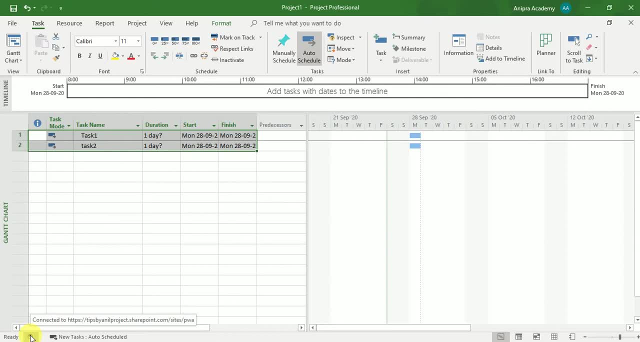 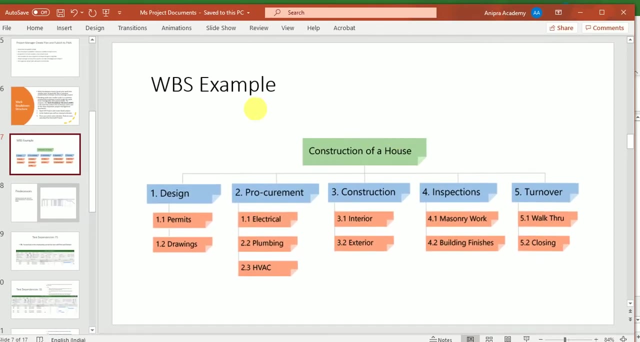 your Microsoft project with PWA. I already discussed in my previous video: Right, so we have to back on work breakdown structure. So if I will take an example you can see over here, WBS example is a construction of a house. It means we have five phases: design, procurement, construction. 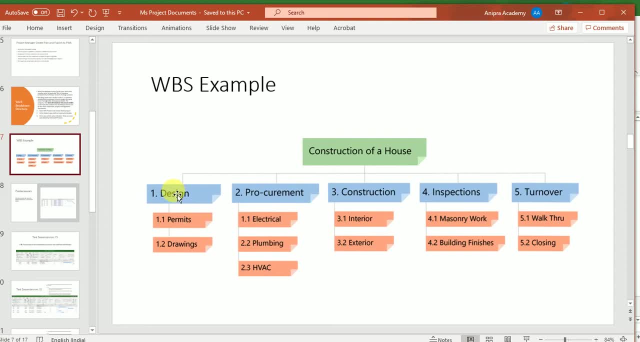 inspection and turnover, And inside every phase we have a different, different task. Like in a design. we have permits drawing in a procurement, we have electrical, plumbing and HVAC right. So how we will break these complete tasks in? 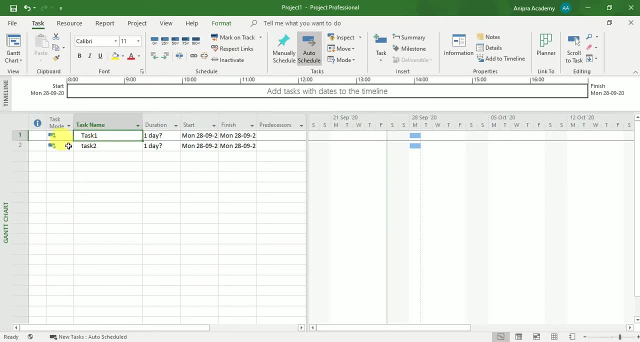 Microsoft project. So just delete these and delete these also. So here I'll say: construction of a house. So this is my project, Construction of a house. This is my project, And under this we have five phases: First it's design, Second is procurement And third is construction causes. 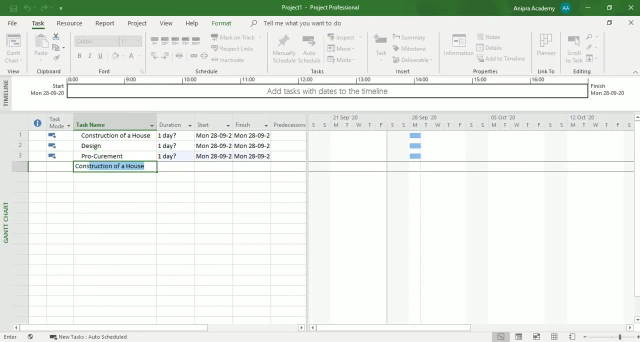 第 3.. And that third is construction. Does the Spelling mistake? still can you please ignore introduction right, void of use, construction Right. and third is inspection. fourth is inspection and the final is turn over. all right, so five phases we have in this. in this project means in this house project. so 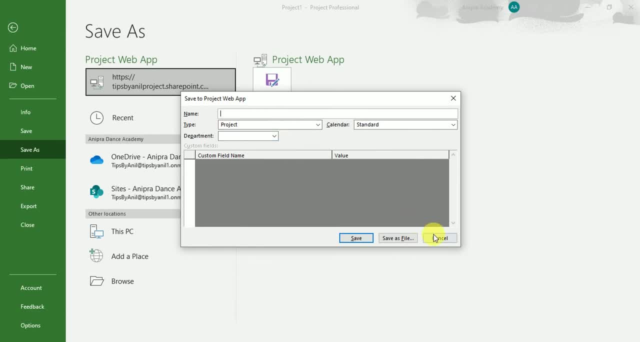 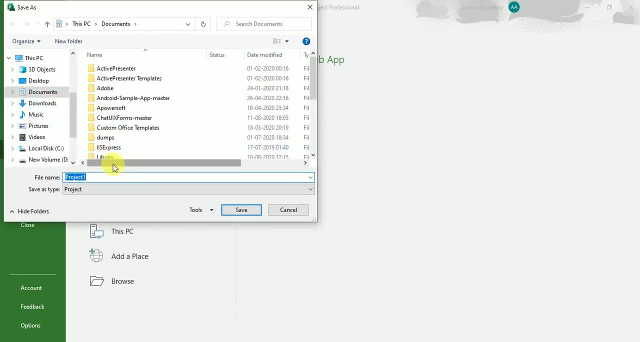 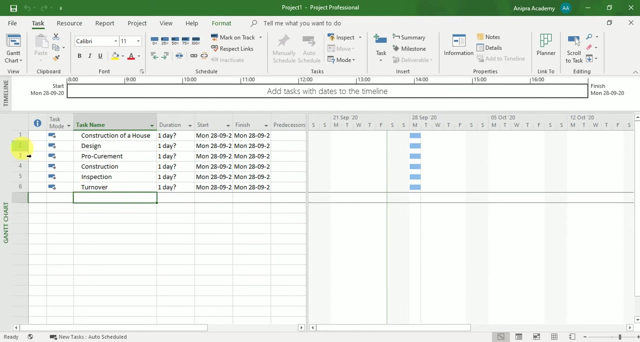 from here. if you want, you can save a project, or either, if you want save it in your local drive, then you can see over here project one: right, it has been saved now inside the design. if I want, I'll just move these as a here you can see. 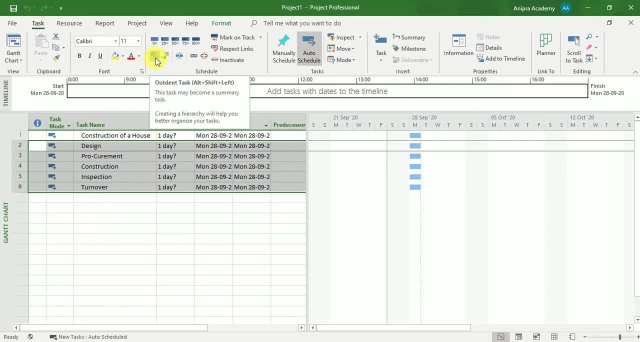 the indent and here you can see the out then. so once you will click on indent, these phases will come under this project, right? so inside this design, if I want to put a task like permits, permits, so this is my task number one- inside the design phase, I'll just do it indent. and the second is: 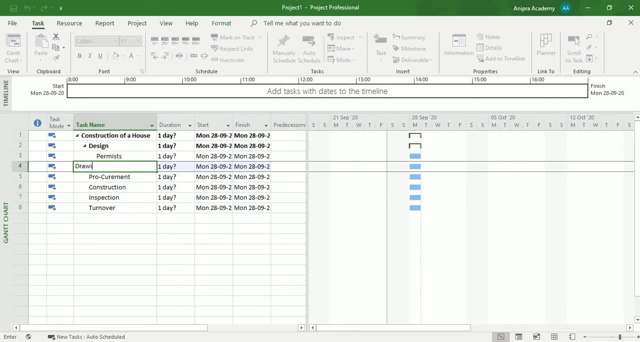 like drawing like. so this is my second task. so if we see from the here indent, I'll shift right, you can just put: I'll shift right also, okay. and now if I'll say in the procurement, then I'll click insert and in the procurement I have two or three. 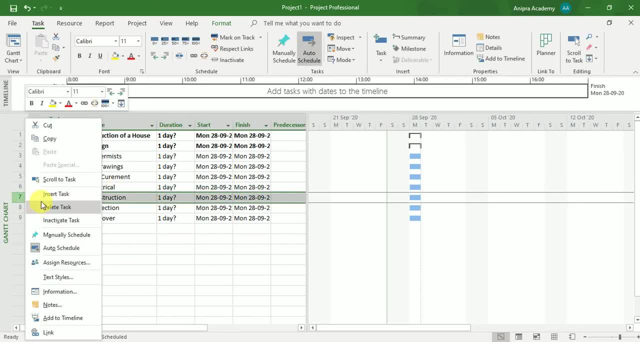 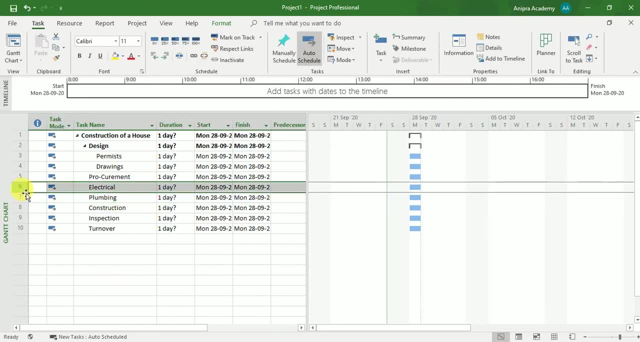 more tasks: electrical and the next is plumbing. okay, so electrical and plumbing, I'll just do the indent. okay, so here, if you will see three phases, in two phases we have tasks and in three phases, suppose, we don't have tasks. okay, so this is my complete work breakdown a. 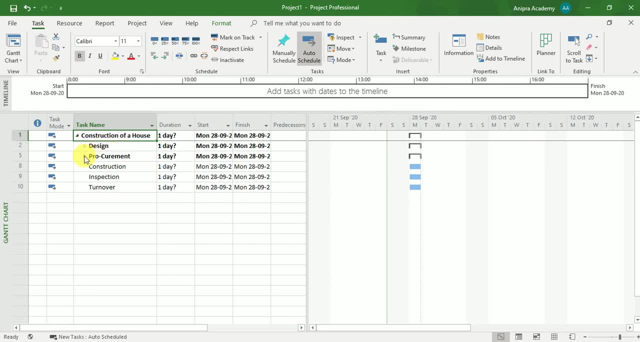 structure for a construction of a house, right? so you are saying these days this is a summary task, basically. so what is the summary task? this summary task is summary of all the phases inside all the tasks, right? so suppose if I'll increase day over here, okay, so you can see the. 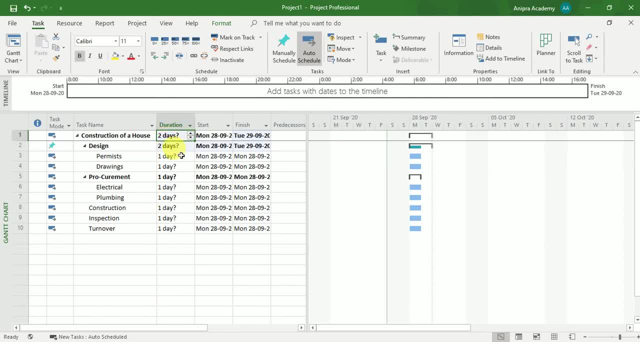 day is automatic increasing over here. what does that mean? we will discuss in my next video in depth. so right now I'll let you know you can see all the phases and then you will go it over to the next two task step- Why it is showing one day or one day and, if I'll change the day over here, why the 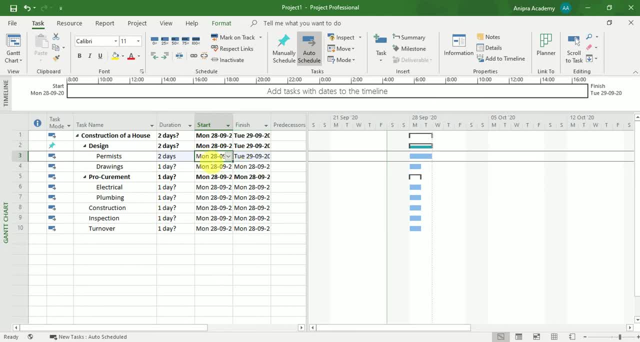 duration of design phase is not going to change because these two tasks are starting parallel. If we'll say this task is starting on 28th of ninth and the same, this task is going to start. so two resources are working simultaneously on this task, but that's why the duration is two days too long. 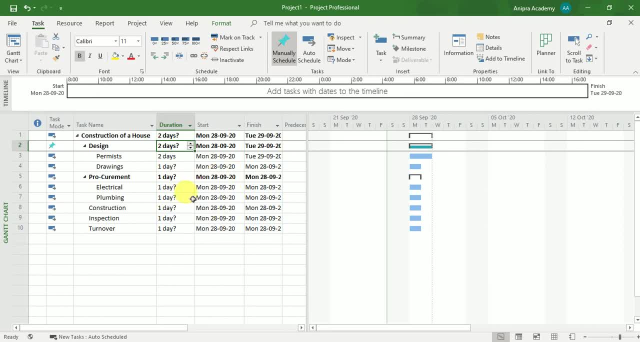 okay, so this is complete work breakdown structure. i hope you like this video and if you like this video, then please subscribe my channel. thanks for watching my video. have a nice day, bye. 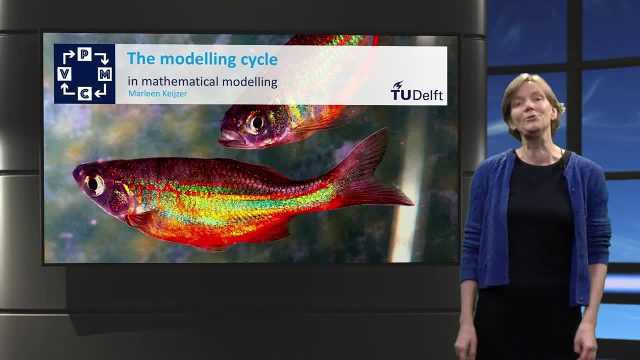 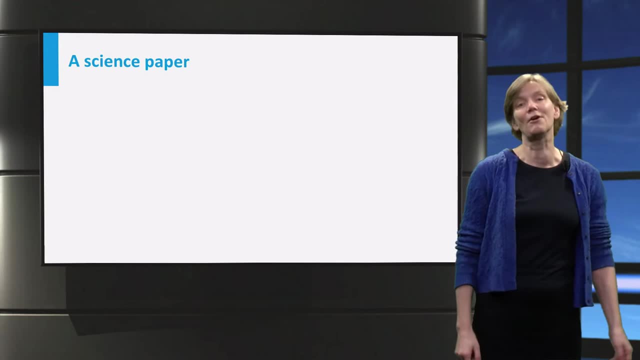 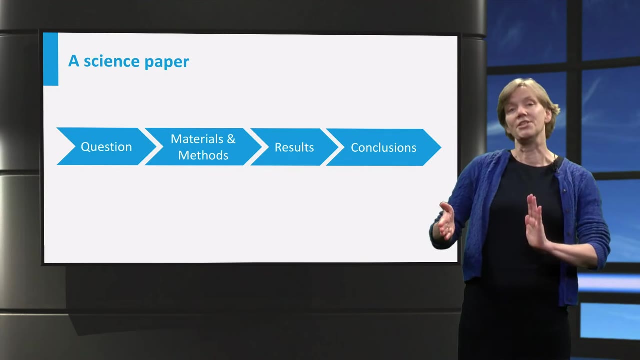 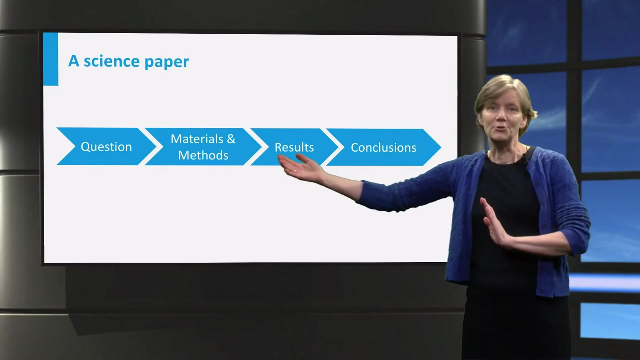 Hi, in this video you learn about the cycle we use when we make mathematical model. In scientific papers, research is often presented as question materials or methods, and then results and conclusions, So a research paper might seem to be a linear process from the question to the answer in one go. However, the path that 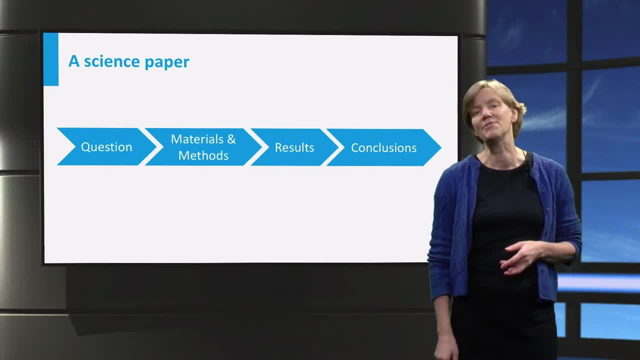 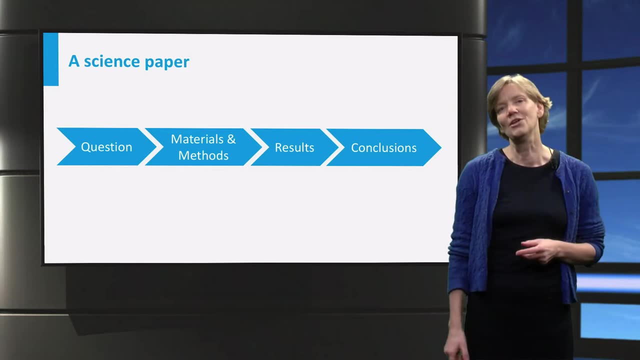 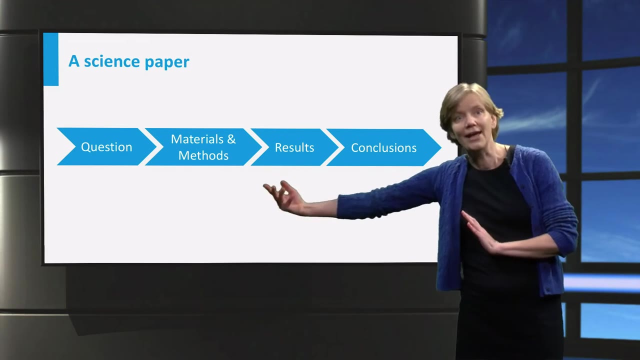 has been followed to obtain those results is almost never linear. By definition, research is new and most often the first results are not good enough or the conclusion does not exactly answer the question you started with. So you have to go back and use a method that is better suited, or you.